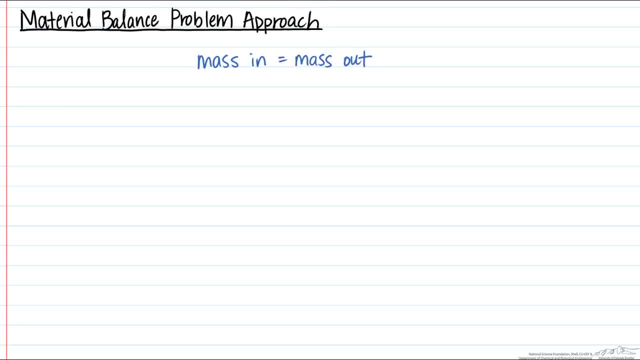 what does the problem ask for? Write it in terms of variables that you set. Read the problem carefully. ask yourself: what do they want? Look for key words or phrases. If you see something like overhead product, then it means that you have product coming out. 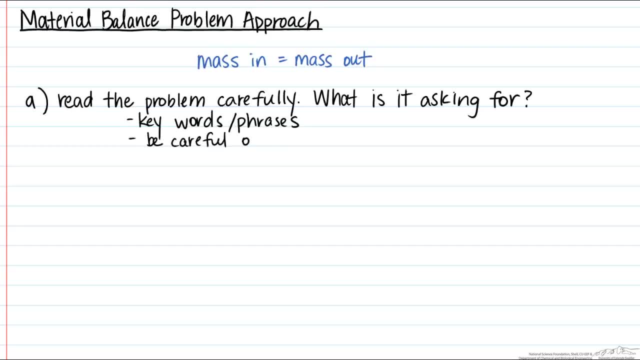 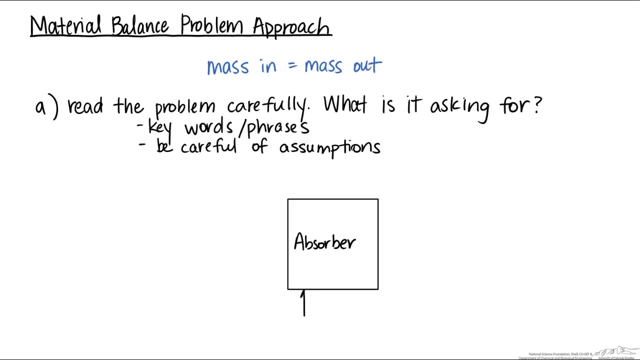 of the top of, perhaps, your column. Be careful of what you assume. Some examples of this are adding streams, leaving streams out, and let me show you a typical example. Let's say we have an absorber, There's a gas stream that comes in and comes out, and a pure liquid enters the. 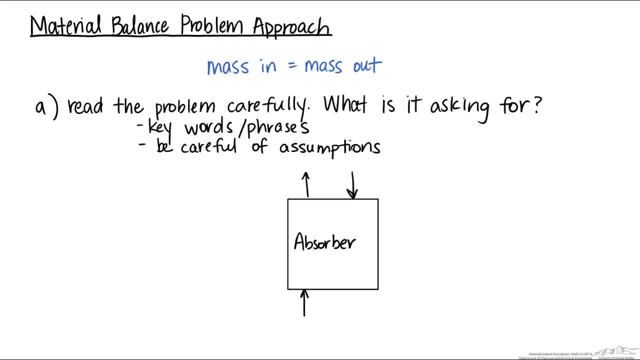 absorber to absorb some of the components of the gas stream. Well, if this stream enters the system, it needs to exit the system. even if the problem doesn't specifically say that there's an aqueous stream exiting the system, It has to come out. 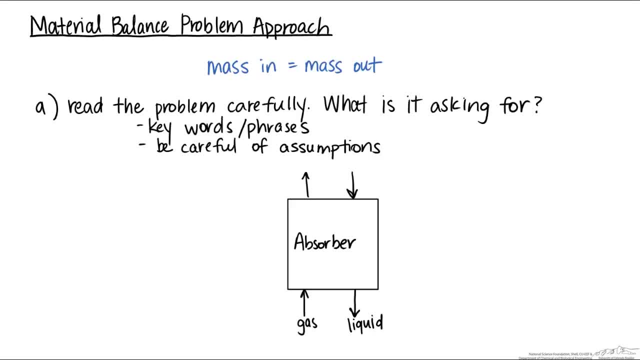 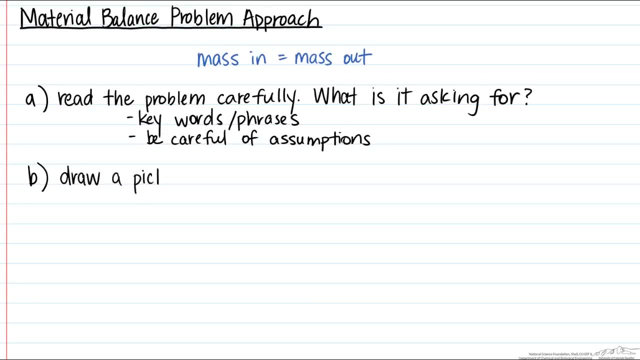 Even if there's a quantum in the system, if the final form of gas that we're studying, if it's not pure- in fact, it probably isn't- because the purpose is for it to pick up some of the components from the gas stream. The next thing to do is draw the picture Label. 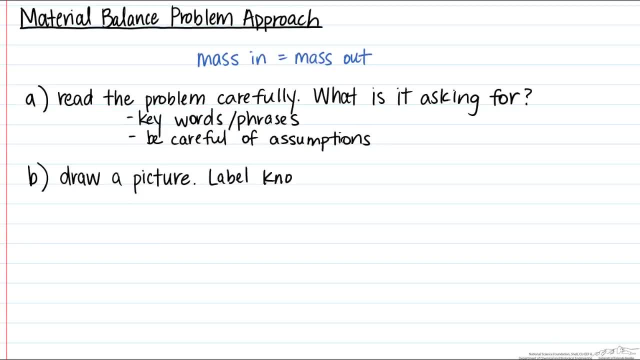 the unknowns and the knowns. What I tend to do is I use m for mass and I use n for moles. For simpler problems, I'll use x for our mass fractions and y for our mole fractions If I'm looking for a particular mass fraction or mole fraction. 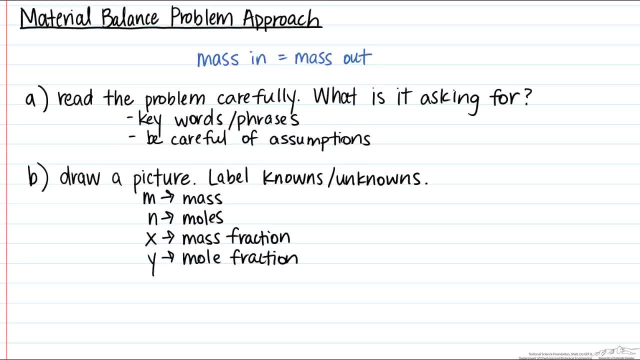 I tend to label it with something that indicates the component. So, for example, if I have a mass fraction of benzene, I'll call this x sub b. Finally, if there's more than one stream that has benzene- let's say there's benzene in stream 2 and in stream 4, I'll write x. 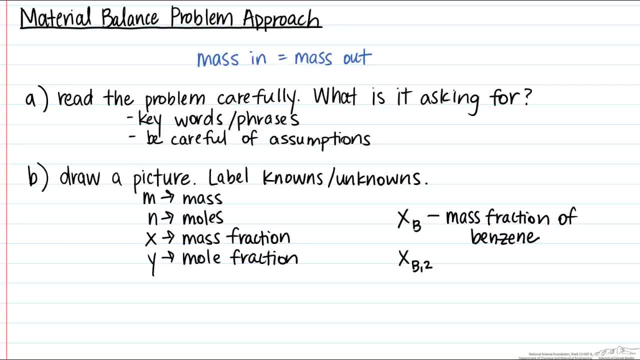 sub b. The more organized you are, the easier it is for you to solve. Another suggestion is to solve for the easy unknowns ahead of time. Don't do major calculations because, first of all, you may end up confusing yourself and, second of all, somebody looking at your 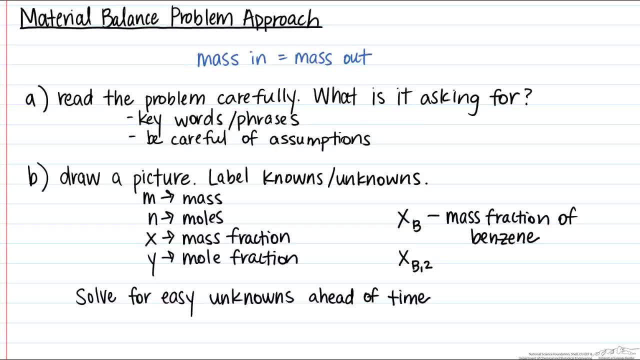 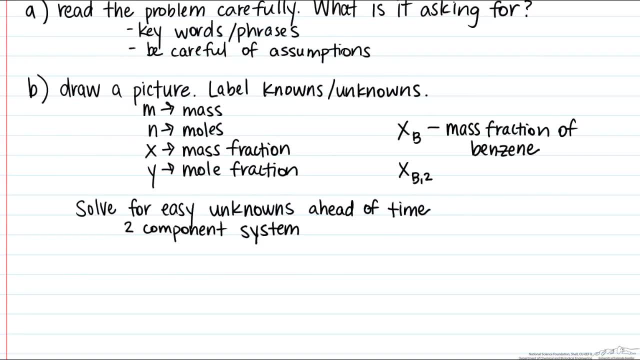 flow chart may not understand how to solve for the easy unknowns ahead of time. That's because there isn't that much evidence that shows that the problem is that your flow chart has mold fraction or one of the two components in your system. This is what you. 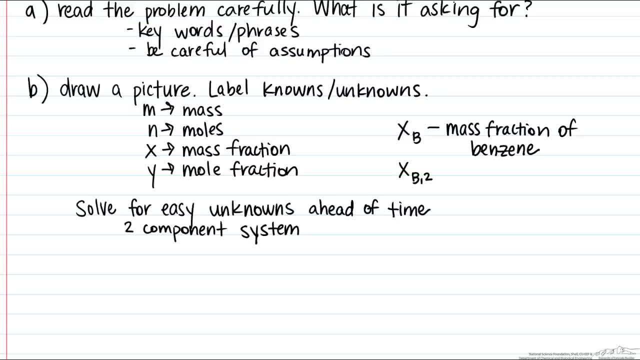 should do. The problem is you have a first and second component system. The problem is that if you have two components in your system, they are every single one. Number 1 is the number 1.. Number 2 is the number And number 3 is the number. So we have to think about. 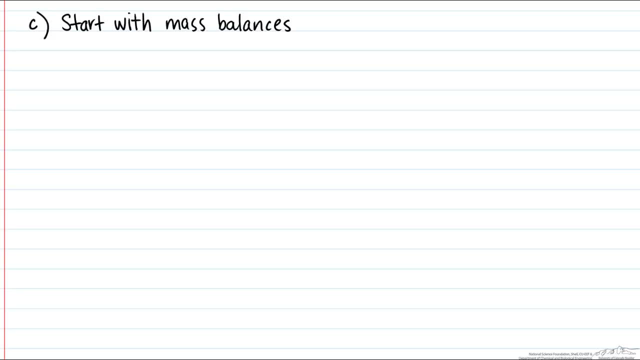 all the factors inside that the material balances, And the thing to remember is that there is one mass balance for every component. One thing that you can do is that you can substitute one overall balance for a component balance, And one of the things that you have to be careful of when you are. 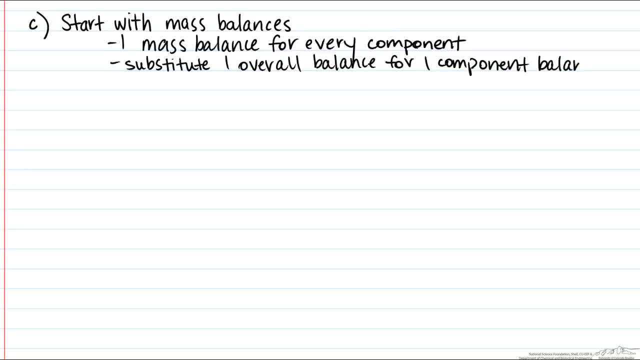 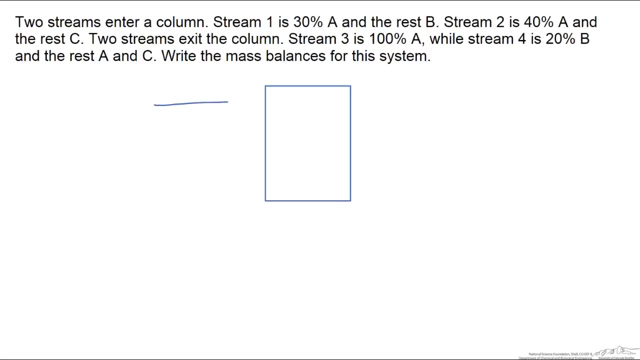 doing your mass balance is that each one of your equations or balances is independent. So let me show you an example. We have two streams that enter a column. Our stream one is 30% A, Okay, And the rest B. There is an example of solving for simple unknowns. Stream 2 is 40% A and 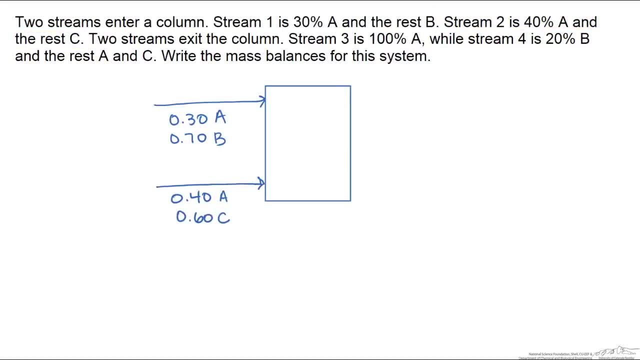 the rest C. So two streams exit the column. Our stream 3 is 100% A And stream 4 is 20% B And the rest A and C, And we are going to write this using the fact that the sum of 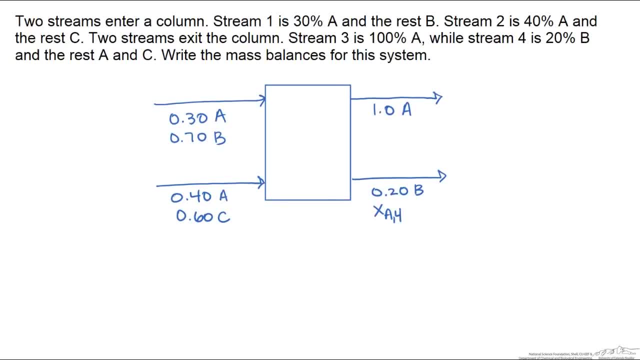 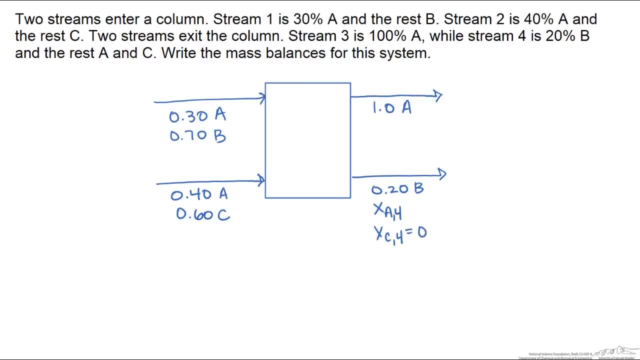 the mole fractions equals 1.. So our X sub C is equal to 0.8 minus X sub A, And we are going to assume that everything is in mass fractions, Okay, And so we need to write the mass or material balances. We will call this M1, M2, M3 and 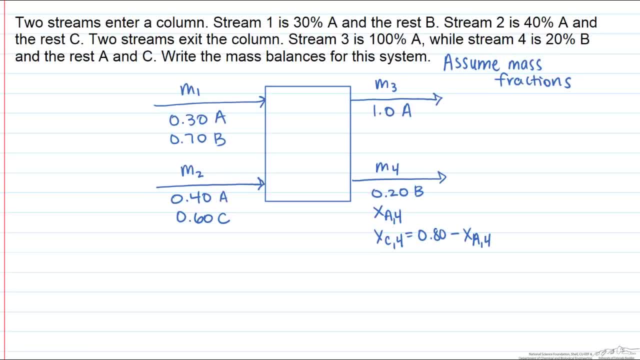 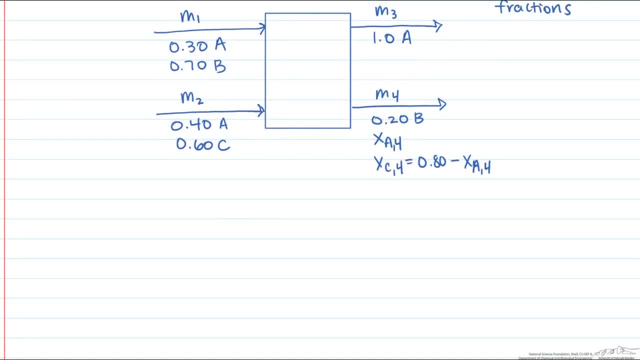 M4.. So now let's do these mass balances And we will start with A. So the amount of A that comes in is 30% of M1.. Okay, So we have 30% of M1 plus 40% of M2. And exiting we have 100% of M3 or just M3 plus. 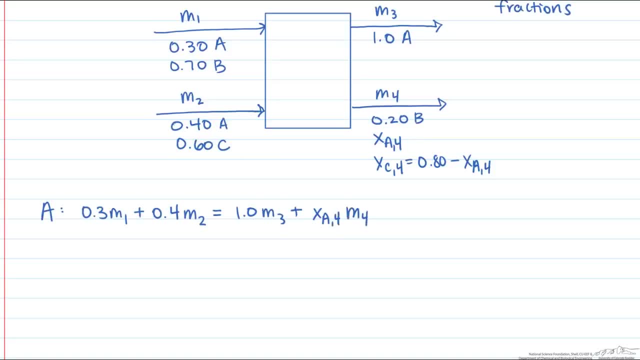 our X sub A times M4.. Now we will do the B balance. Coming in the first stream, 70% is M1.. There is nothing in M2.. There is nothing in M3. It is 20% of M4.. Now our C balance. 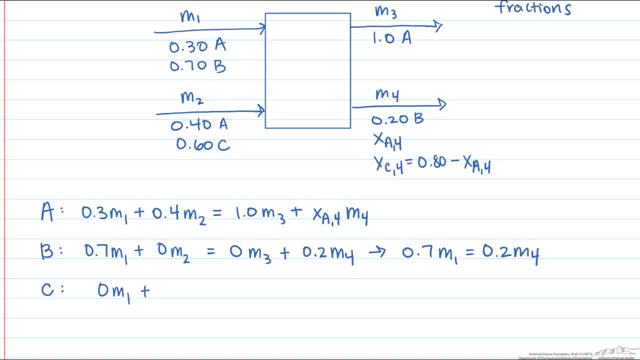 which nothing is in M1. C is 60% of M2. And coming out we have 0.8 minus M2. So we have 0.8 minus X sub A times our M4.. These are our three component balances. Let's see what happens if we add them all together. 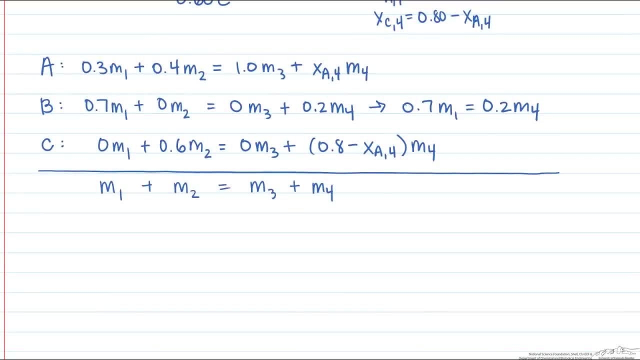 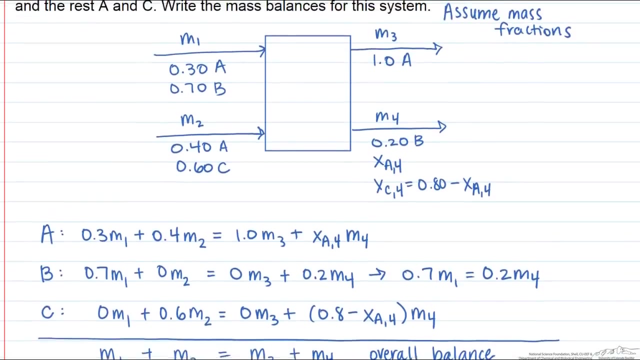 So note, when we add them all together, what we get is the overall balance. So we can only use 3 out of these. Okay, Okay, Okay, Okay, Okay. So you can't solve these four equations to solve our system. Finally, note that we have: 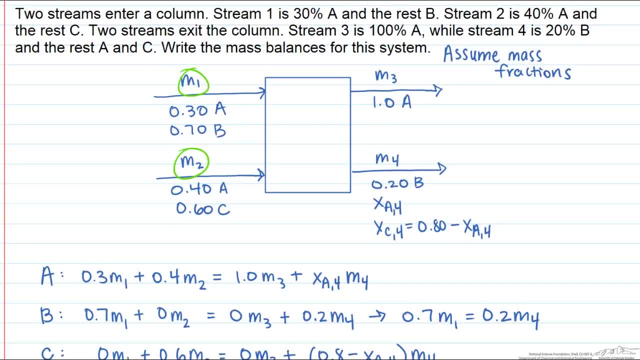 1,, 2,, 3,, 4,, 5, unknowns- but we only have 3 mass balances that we can write. So, as this system is stated, we can't solve it. This is what's called a degree of freedom. Now,